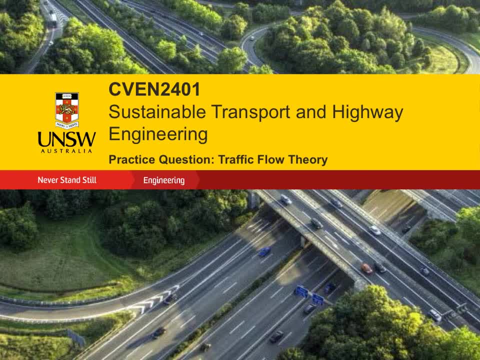 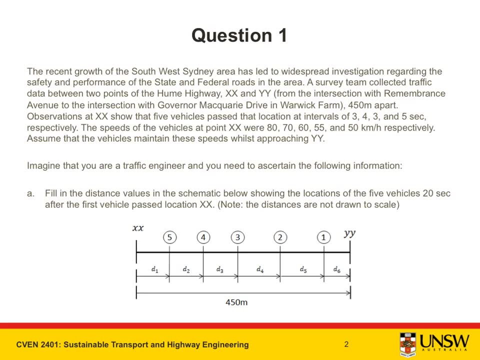 This video walks through a practice question on traffic flow theory. As I read through the question, I'll highlight any key terms and information so that we can easily identify and refer back to these later. The recent growth of the South West Sydney area has led to widespread investigation regarding the 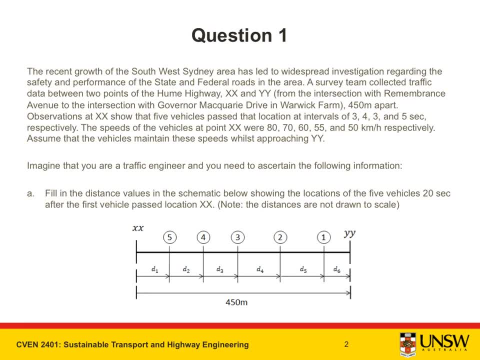 safety and performance of the state and federal roads in the area. A survey team collected traffic data between two points of the Hume Highway XX and YY, from the intersection with Remembrance Avenue to the intersection with Governor Macquarie Drive in Warwick Farm. 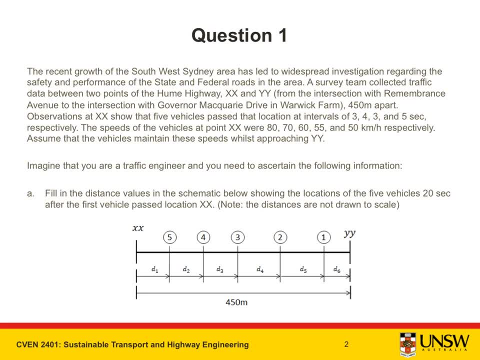 450 metres apart. The speeds of the vehicles at point XX were 80,, 70,, 60,, 55 and 50 km per hour respectively. Assume that the vehicles maintain these speeds whilst approaching YY. Imagine that you are a traffic engineer and you need to ascertain the following information. 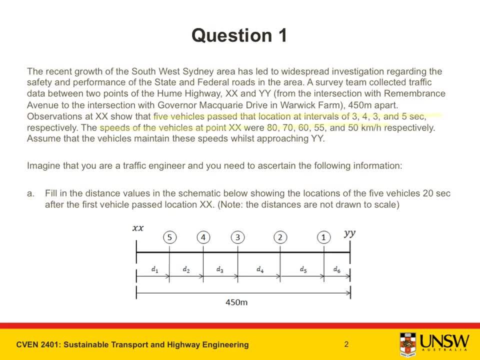 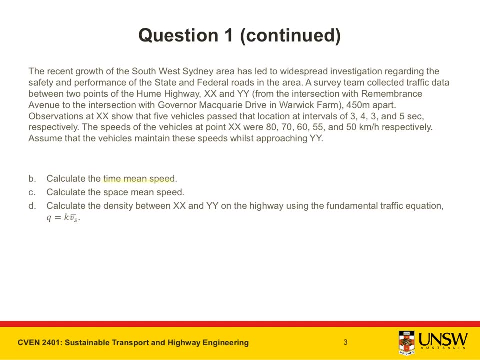 Part A: Fill in the distance values in the schematic below showing the locations of the five vehicles 20 seconds after the first vehicle passed location XX. Part B: Calculate the time mean speed. Part C: Calculate the space mean speed And finally, Part D: Calculate the density between XX and YY on the highway. 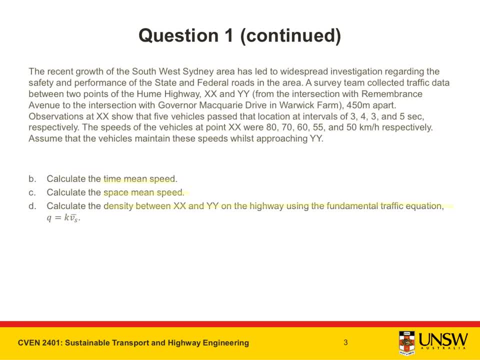 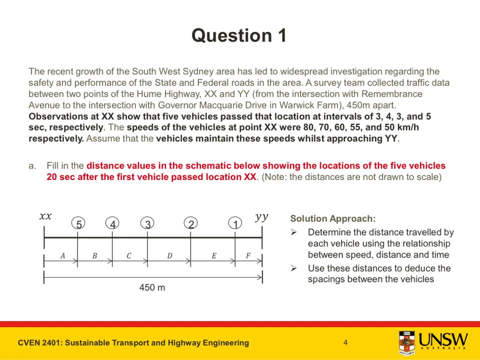 using the fundamental traffic equation, Q is equal to KVS. Let's now take a closer look at Part A. We are given a schematic diagram showing the locations of XX and YY and need to determine where the vehicles are 20 seconds after the first vehicle passes. location XX: 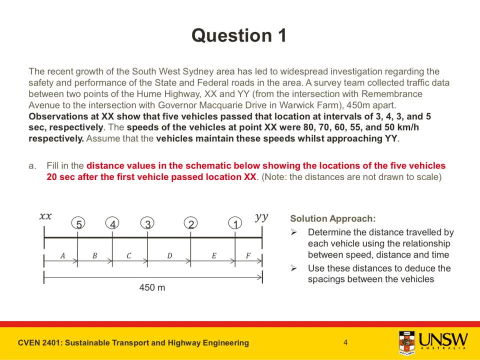 To do this, we first calculate the distance travelled by each vehicle using the relationship between speed, distance and time, and then use these to infer the spacings between each vehicle as required by the question. Recall that the distance travelled by each vehicle is equal to the distance travelled by the vehicle. 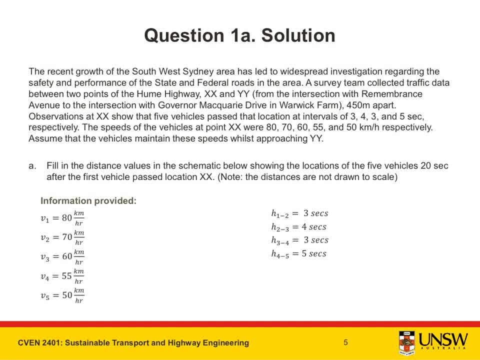 By recapping the information that has been provided. we are given directly the speed of each vehicle in kilometres per hour. We will need to convert these speeds to SI units, that is, metres per second. The time interval between each vehicle passing XX is given as well. 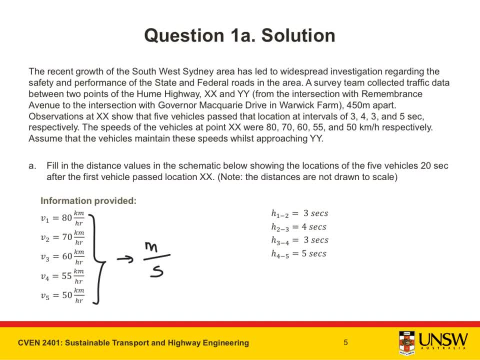 This is called the headway. For example, after vehicle 1 arrives at XX, 3 seconds elapses before the following vehicle. For example, after vehicle 1 arrives at XX, 3 seconds elapses before the following vehicle, Vehicle 2, arrives at the same point. 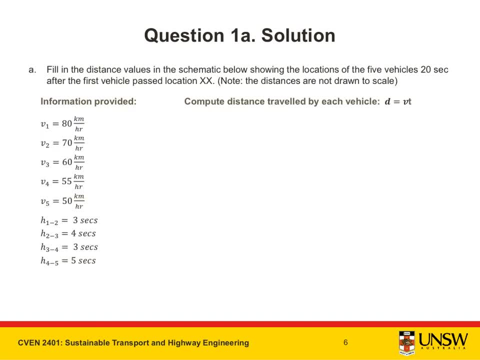 Vehicle 2 arrives at the same point. Let's now compute the distance travelled by each vehicle after 20 seconds has passed. using D, the distance is equal to V, the speed multiplied by T time For vehicle 1,. the distance travelled is equal to the speed 80 kilometres per hour converted into metres per second. 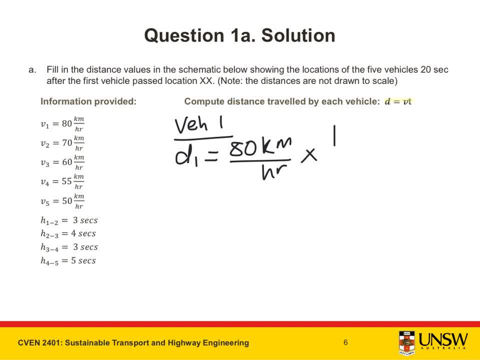 For vehicle 1, the distance travelled is equal to the speed, 80 kilometres per hour. converted into metres per second. The distance travelled is equal to the speed reliefula- varied by the distance travelled. so speech multiplied by the time, which is the entire 20 seconds. since it is the first vehicle to pass XX. 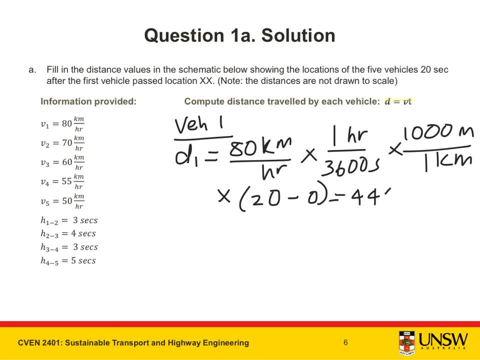 This gives us 444.44 meters, adequate maximum critical For vehicle 2,. the distance travelled is equal to 70 km per hour converted into meters per second, once again multiplied by the time, which is 17 seconds, since the second vehicle passes XX three seconds later than the first vehicle. 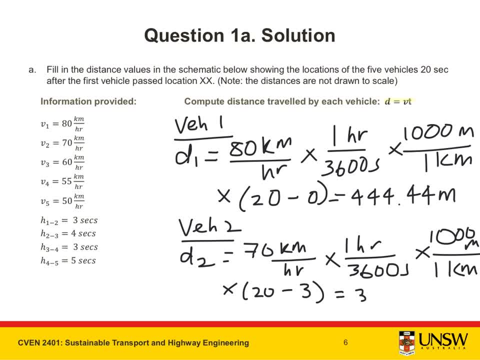 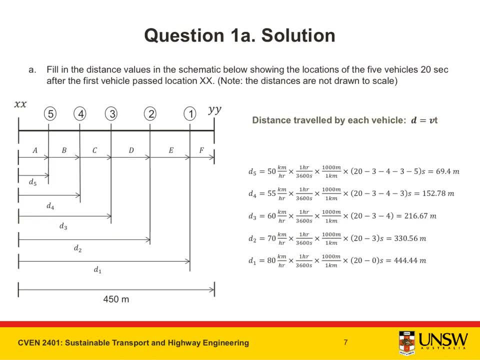 This gives a distance of 330.56 meters Subtitles by the Amaraorg community. Applying a similar procedure to vehicles 3 to 5 yields the following results: As you can see, vehicles arriving at XX at later times do not travel as far along the XX to YY interval. 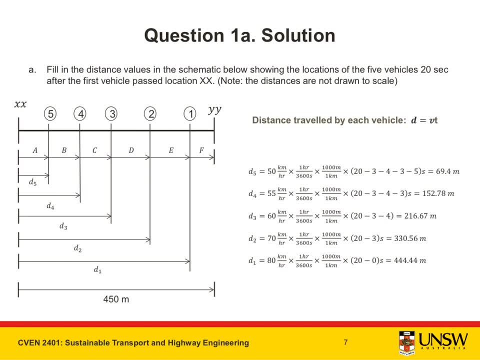 For example, vehicle 4 only reaches a distance of 152.78 meters and vehicle 5 reaches a distance of 69.4 meters. Subtitles by the Amaraorg community. Now we can use these distances to determine the spacing between each vehicle. 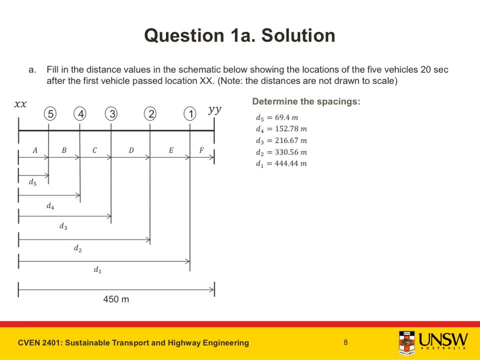 A is simply the distance travelled by vehicle 5, which is 69.4 meters. You can calculate the distance B by deducting D5 out of D4, which gives you a value of 83.3 meters. Subtitles by the Amaraorg community. 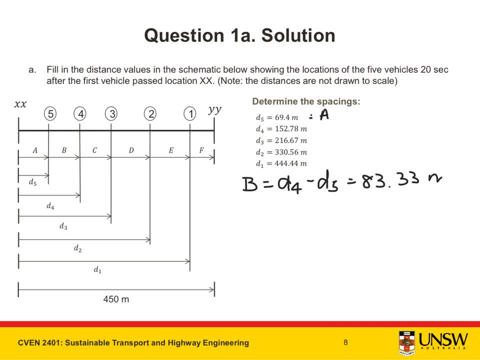 Similarly, we can infer the length of C using D3 and D4.. D, E and F can be found in the same way. Subtitles by the Amaraorg community. Subtitles by the Amaraorg community. Subtitles by the Amaraorg community. 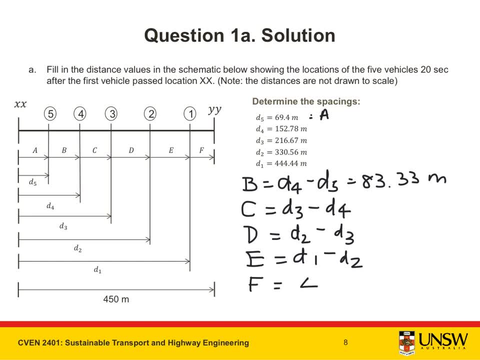 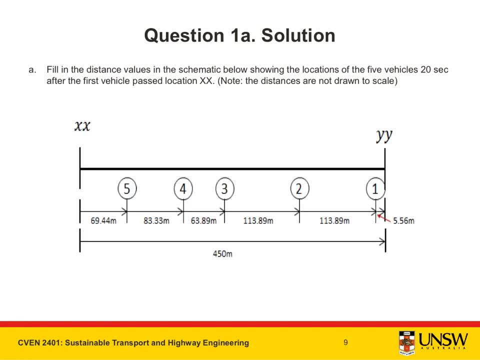 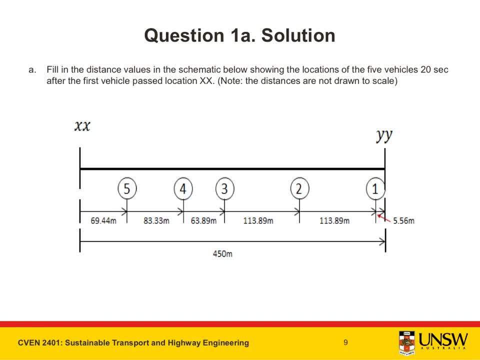 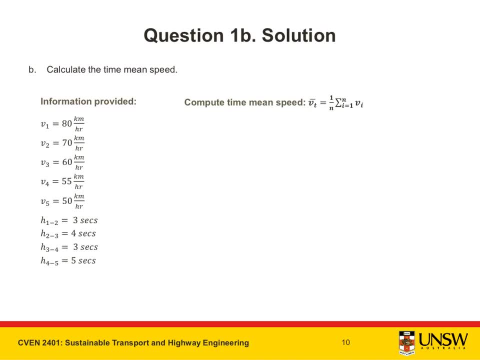 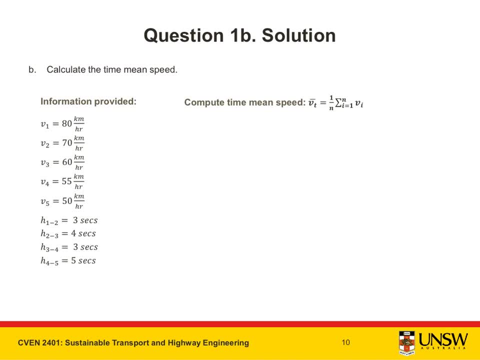 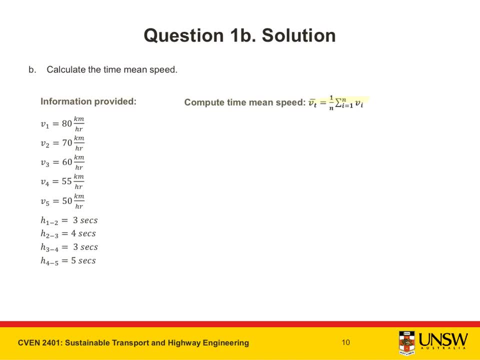 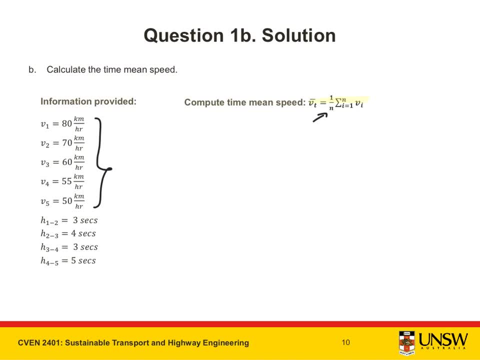 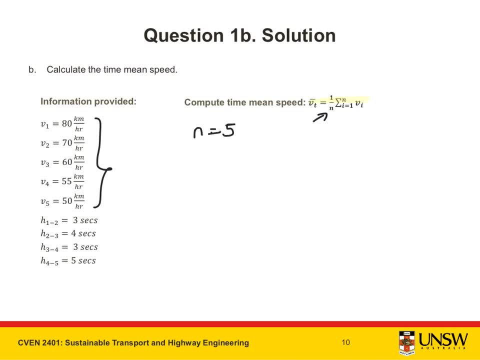 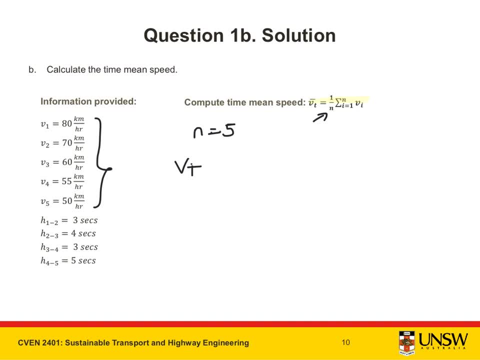 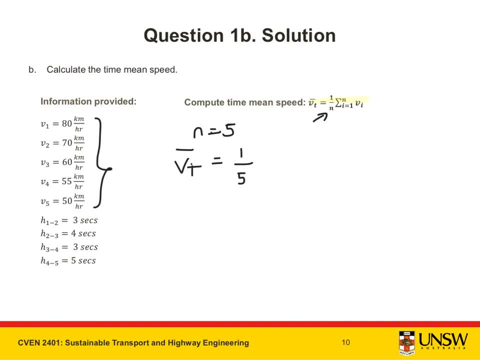 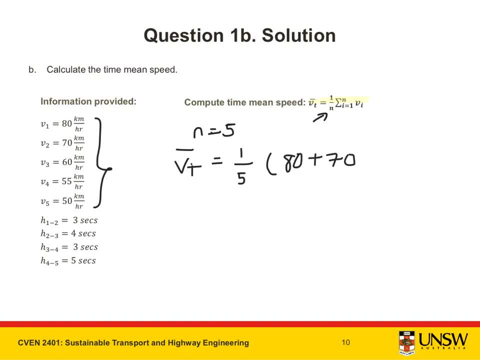 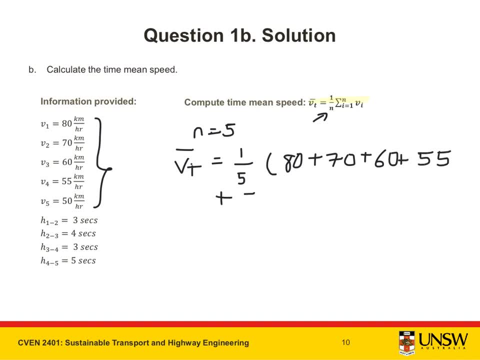 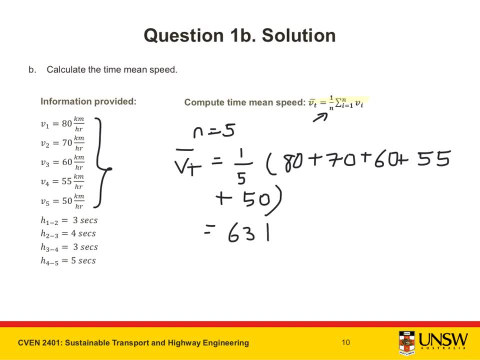 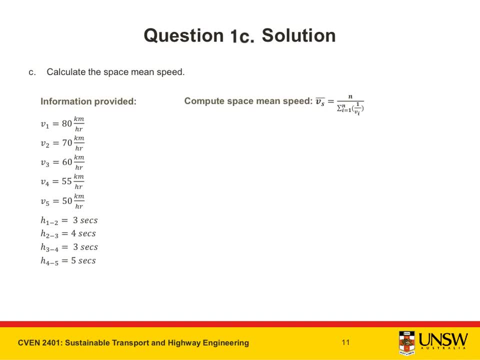 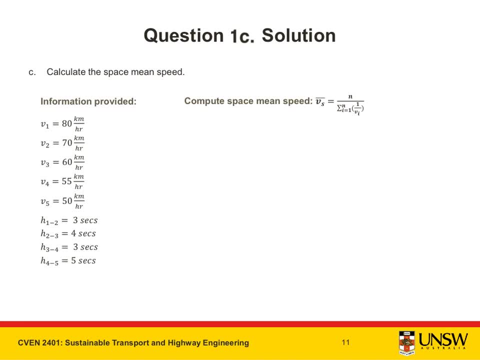 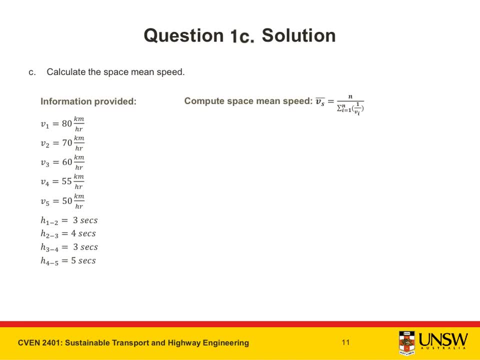 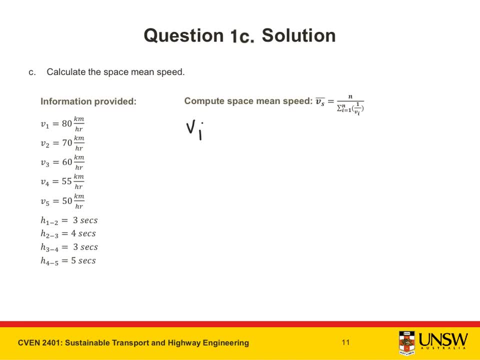 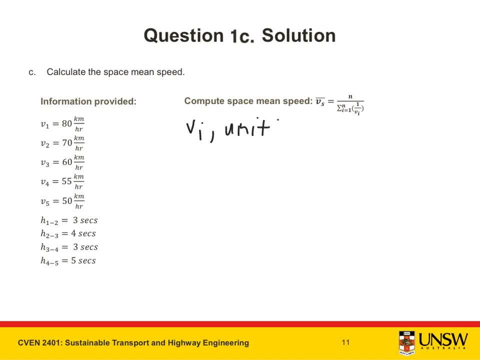 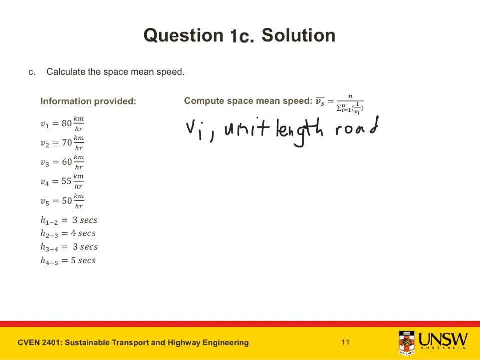 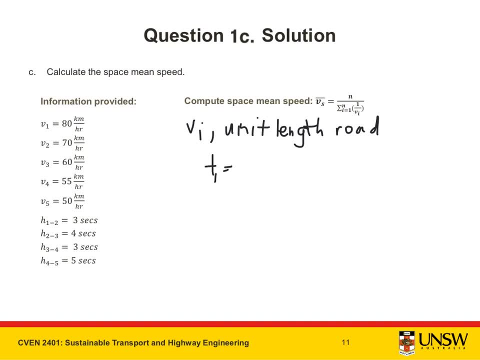 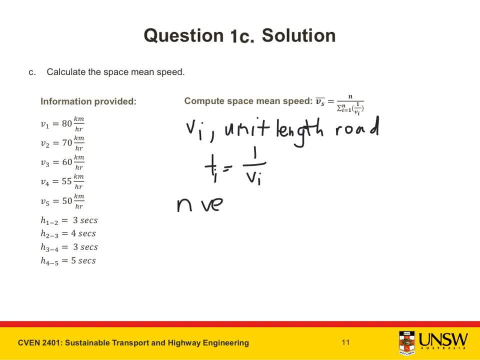 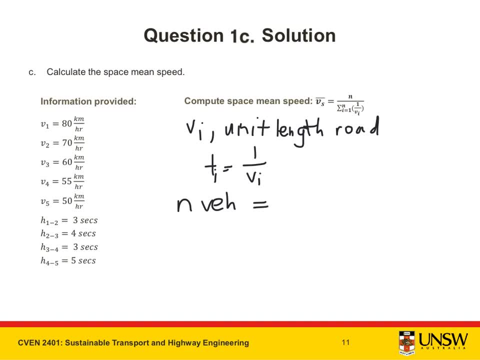 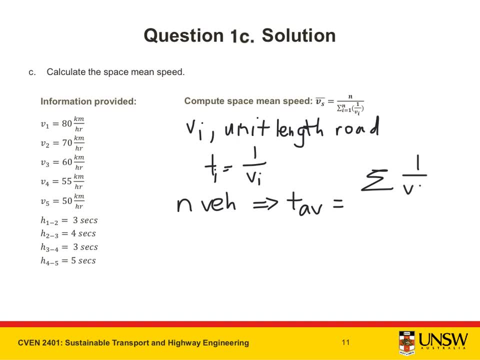 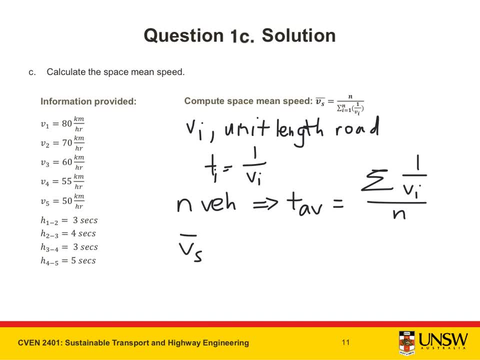 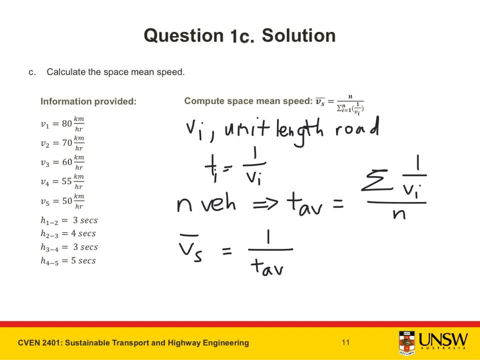 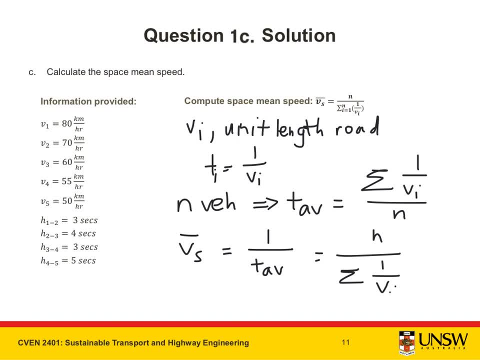 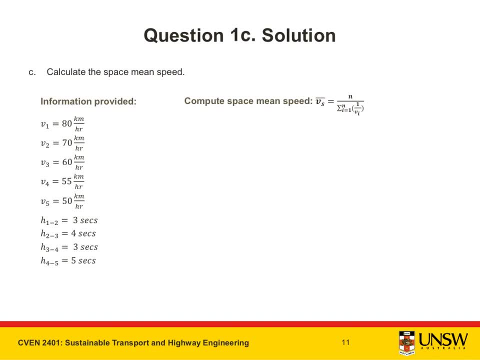 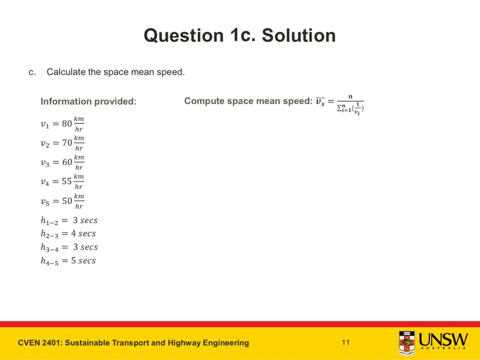 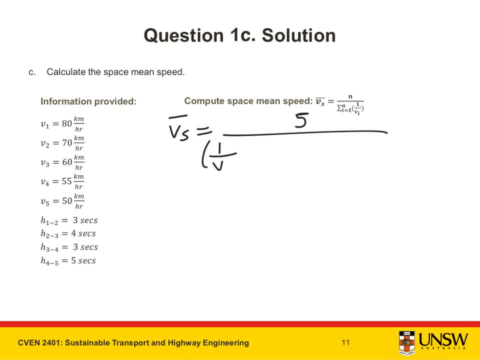 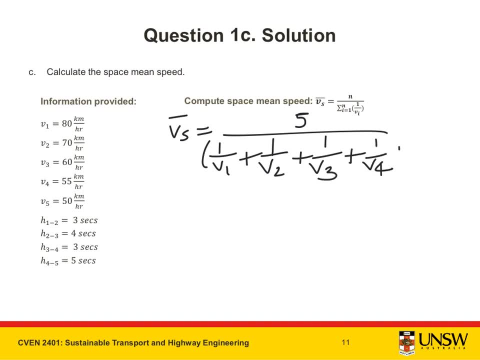 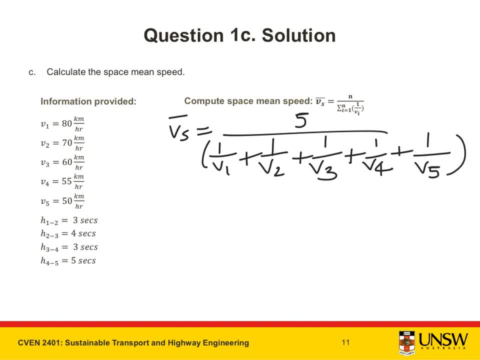 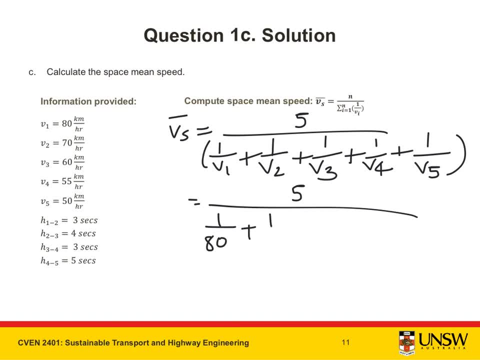 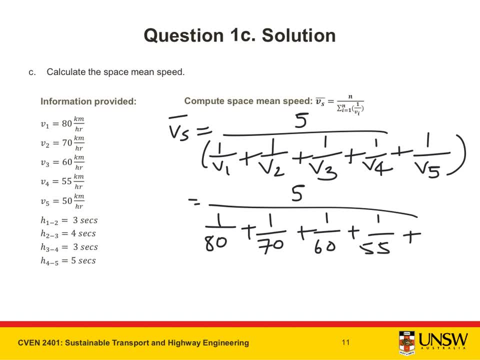 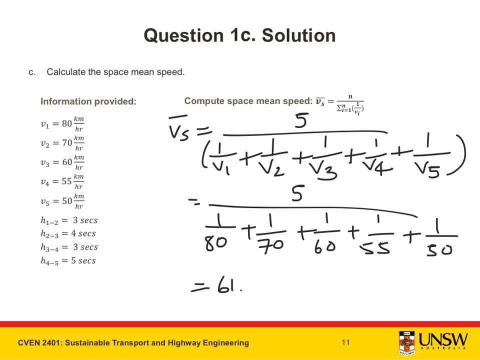 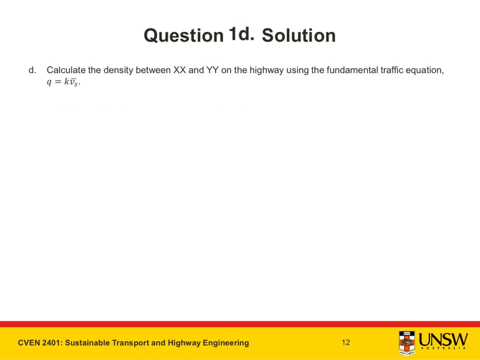 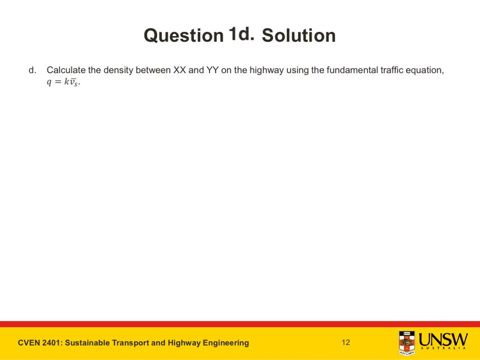 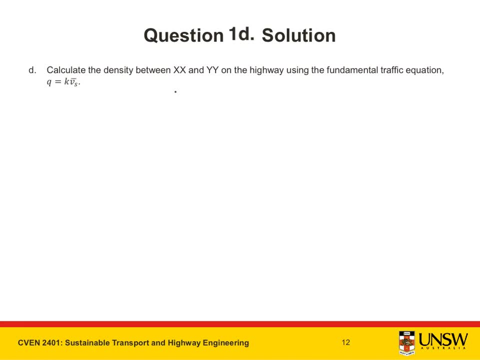 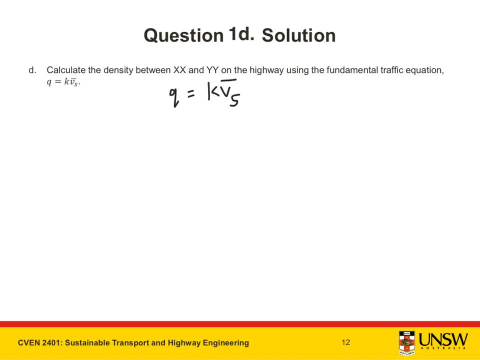 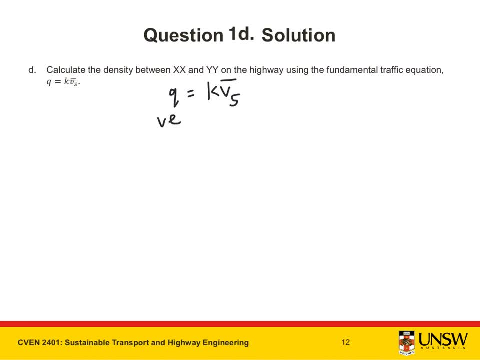 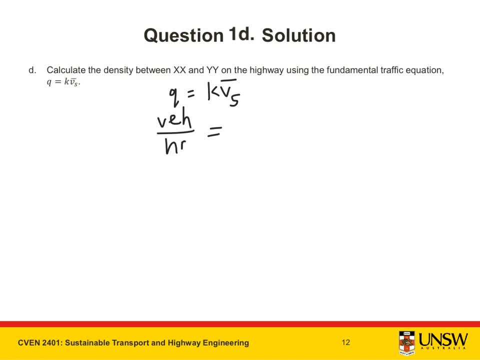 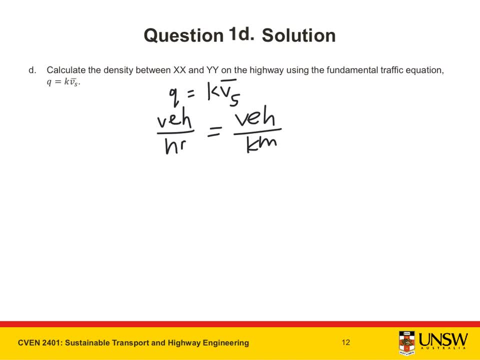 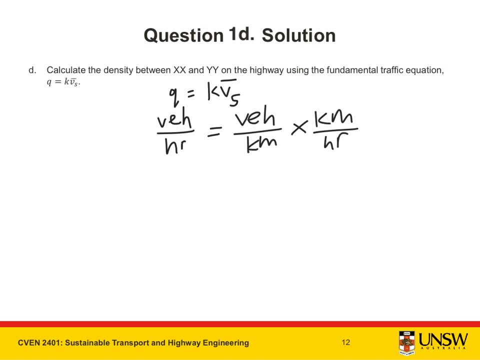 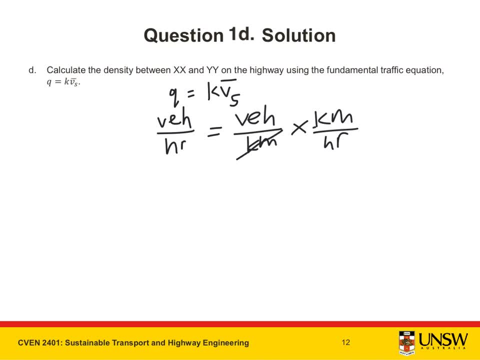 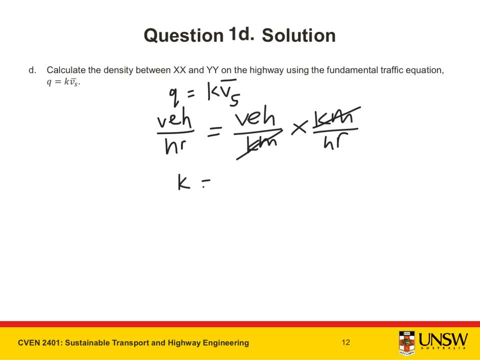 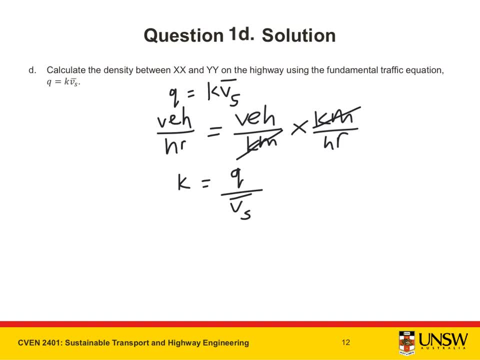 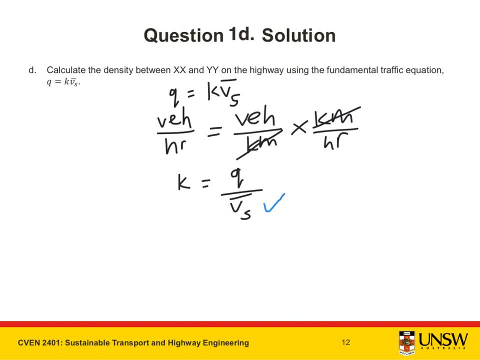 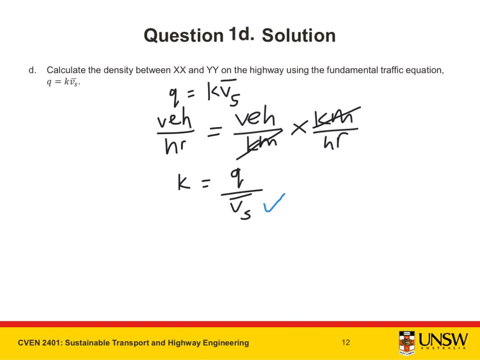 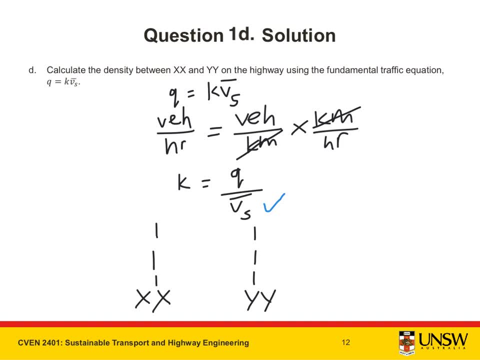 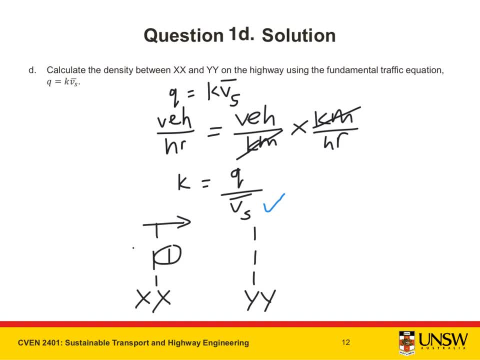 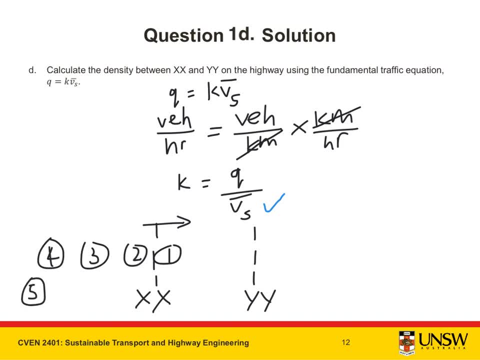 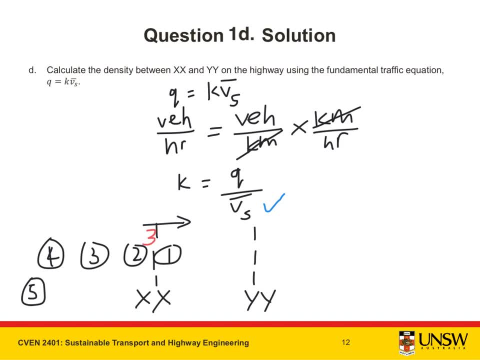 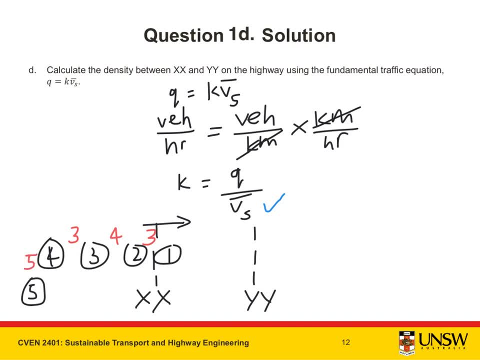 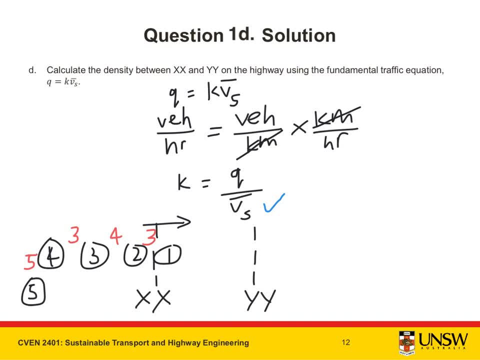 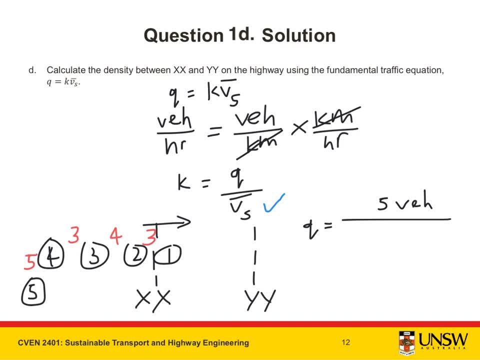 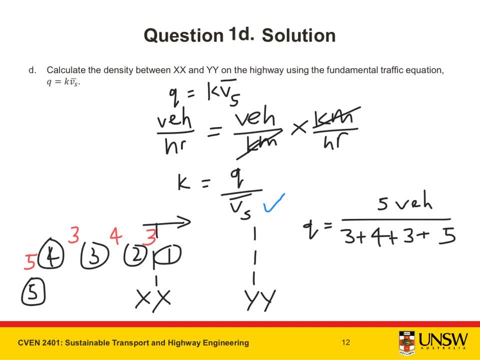 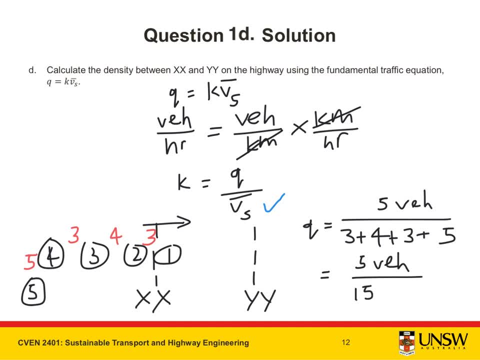 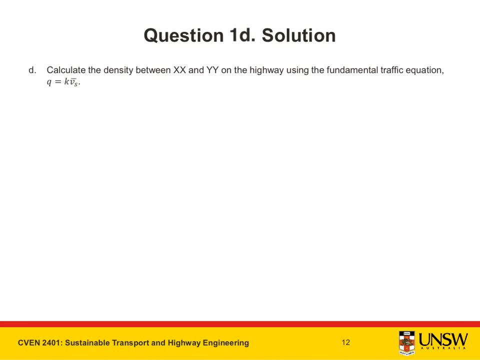 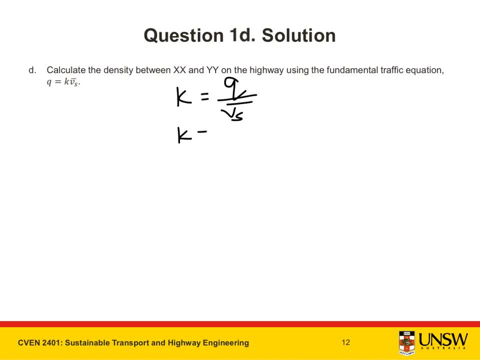 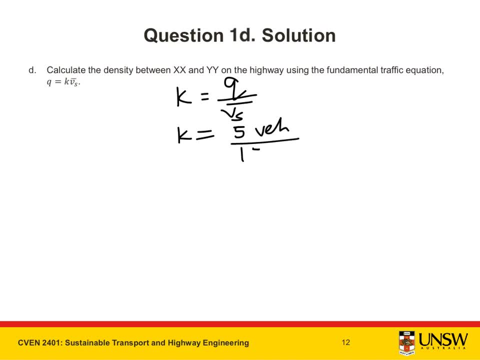 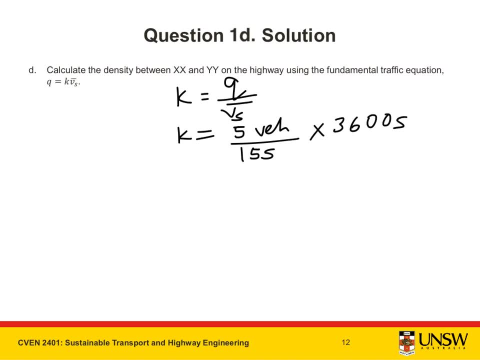 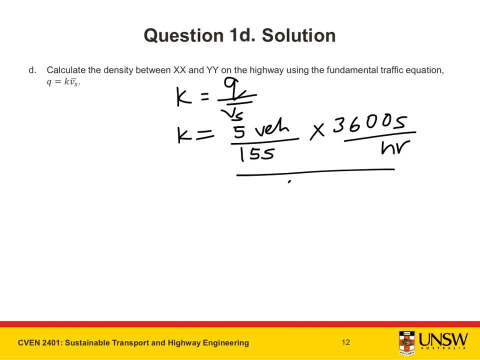 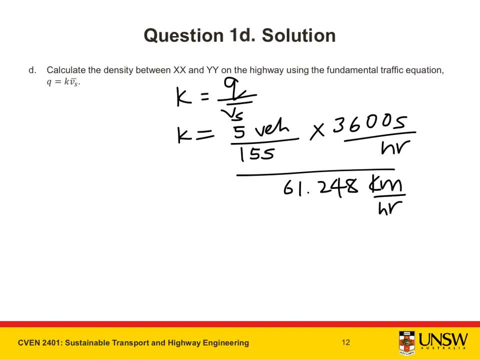 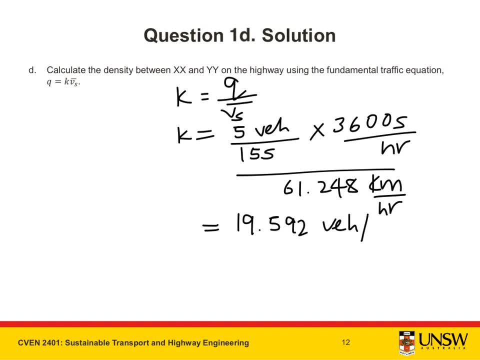 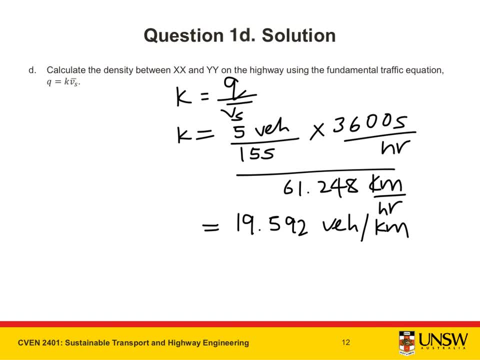 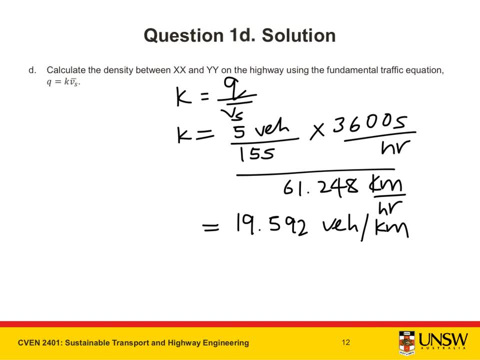 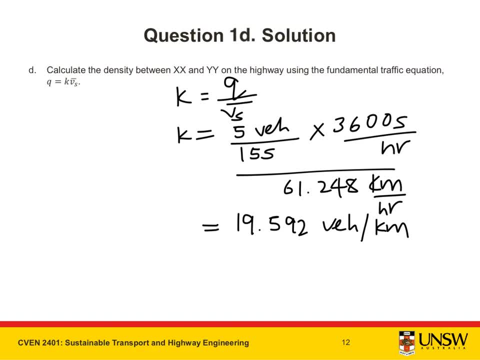